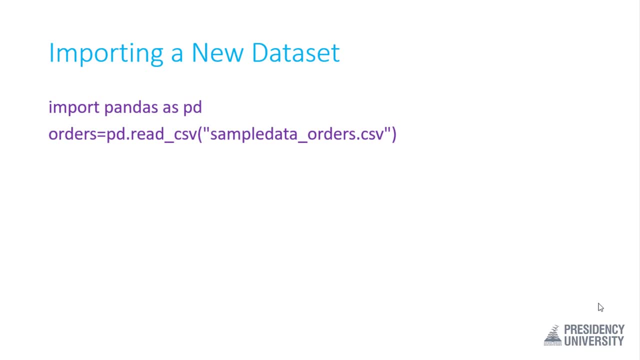 dataset. In order to import a new dataset, we use the library called pandas, using the method import pandas as pd, and we use the method read underscore csv for reading the dataset. Here we have used the dataset sample data underscore orders and we have saved it into 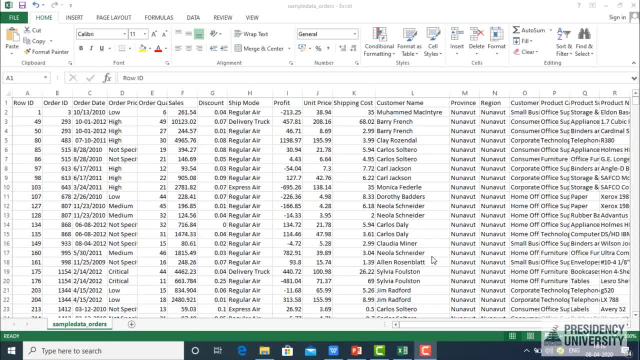 a variable called orders. Let us visualize this particular dataset which we have recently imported. If you can see, there there are different columns, in which the first row contains the column title. We have row id: order: id order, date order, priority order, quantity, sales discount. 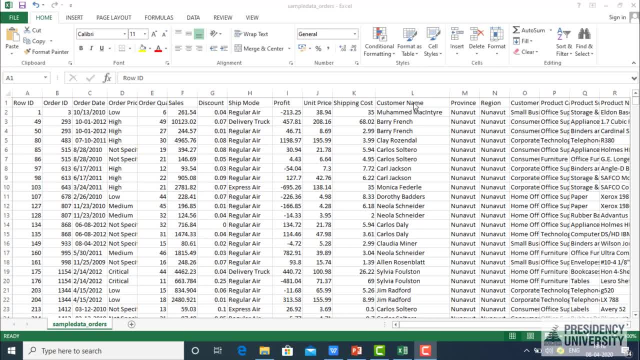 shipping mode, profit unit, price, shipping cost, customer name, province, region and so on. Same way, we also have rows in which we have values for each element, and this is called the indexing of the dataset. So this particular is called the data frame, wherein there are a number of rows and columns. 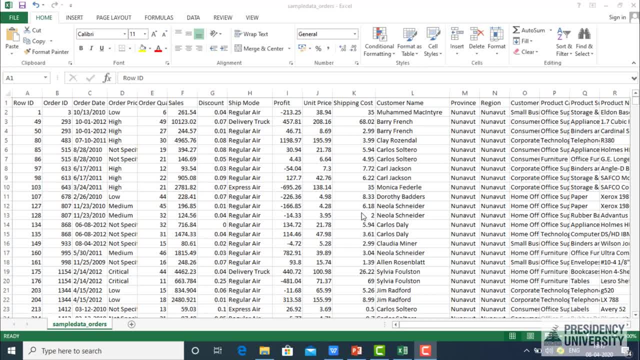 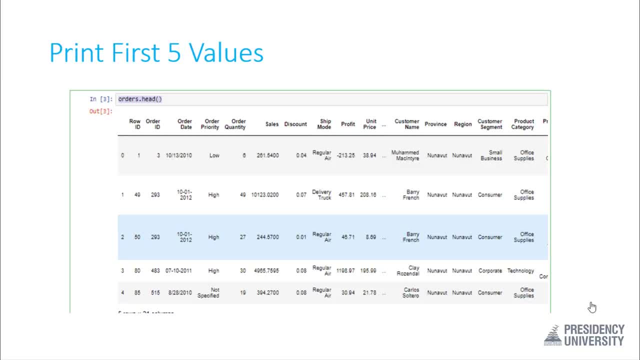 which are specified. We are going to work this. we have imported this into pandas library and we have created a data frame there by the name orders. As you would have seen in the excel sheet, we had the first row as the column title and 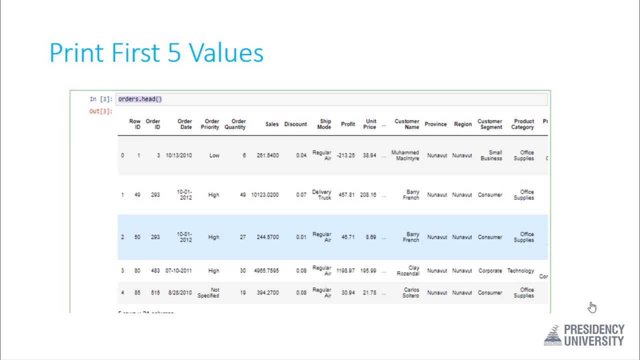 we have had values in the consecutive rows. By default, pandas takes the first row as the column heading or the feature heading Right, And the other rows are taken as the values. And if we have to visualize the first five rows then I use the method called dot head. 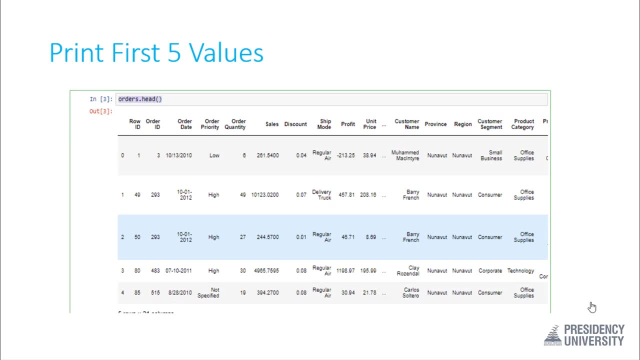 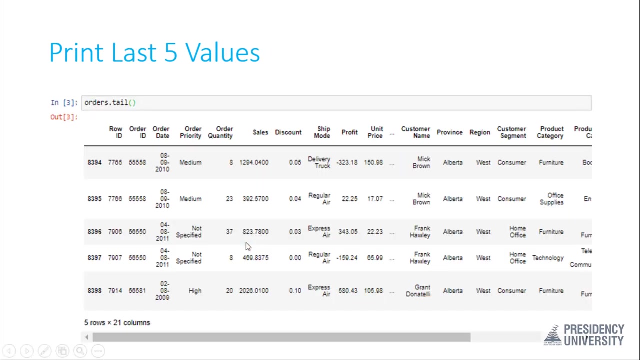 Here, orders is the data frame and dot head is the method to display the first five values. And, as you see, there the first five rows of the excel sheet are displayed as a data frame. In order to visualize the last five values in the data frame, I use the orders dot tail. 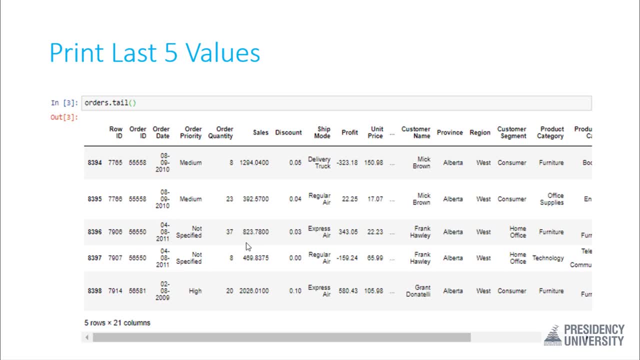 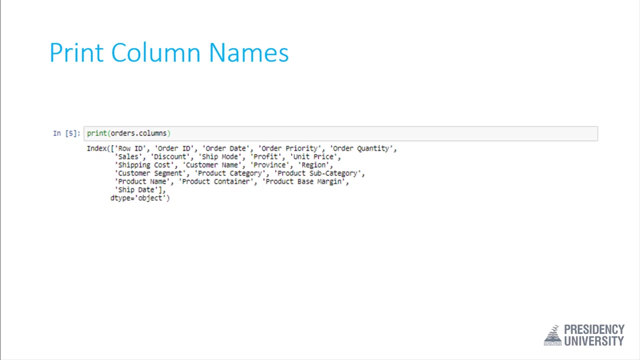 method. The tail is the method to display the last five values. If I want to print the last ten values then I specify orders dot tail of ten. The print orders dot columns method is used to print all the column names Here: row, id, order, id order, date order, priority order, quantity, etc. are all the column names. 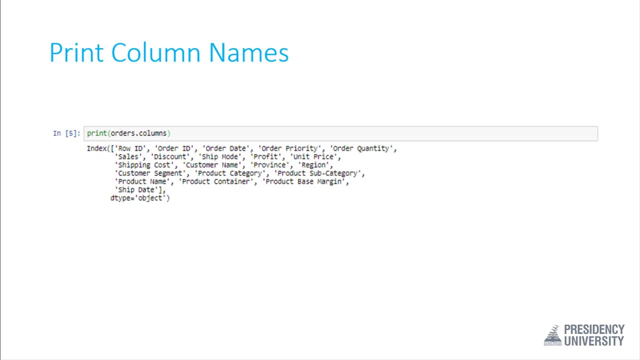 This will help us to get an idea about the columns available in the data frame. Next, we will move on to the next step. Next, we will move on to data sorting. Data sorting is the process of sorting the data in a particular order, as we want. 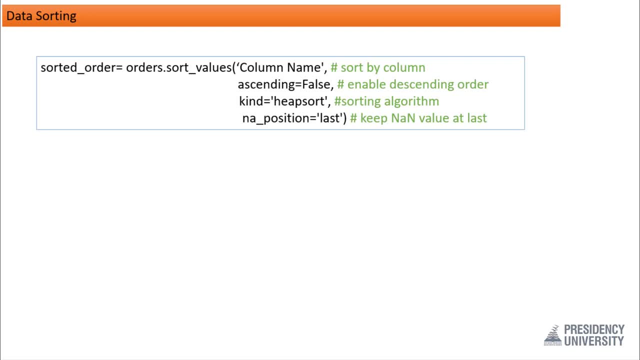 In order to sort values in pandas, we use the sort underscore values method. Here. it takes four parameters. The first one is the column name. The column name is the name of the column which has to be sorted, And we set the ascending to be either true or false. 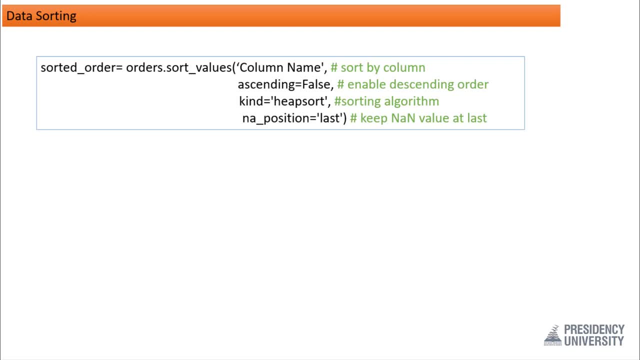 True is for ascending, false is for descending. We also specify the kind of sorting. Here heap sort is used. You can try with other sorts, like bubble or quick, or insertion and so on. And the last one is the NA position. NA is for null values or not a number values. 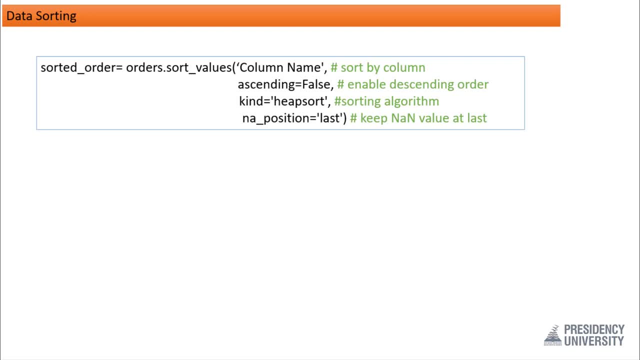 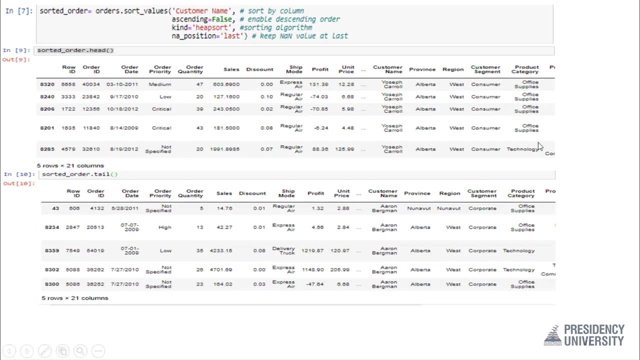 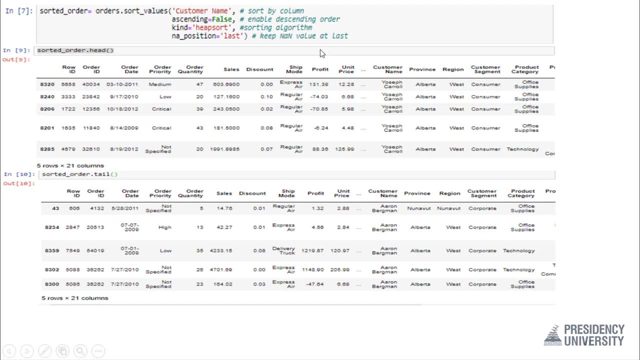 The column name called customer name is taken. I have set the ascending to be false. It means that all the values are going to be in descending order. The type of sort used is heap sort and all the null values are pushed to the last. 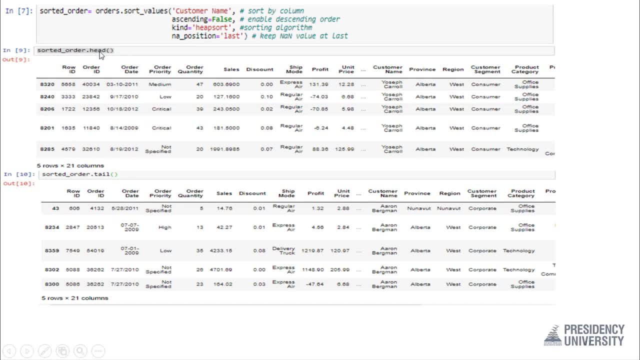 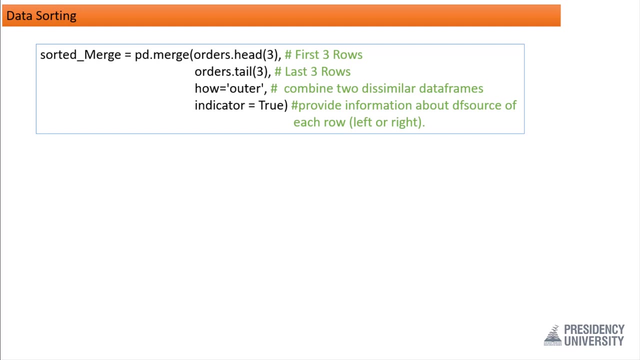 And when I visualize the first I values and the last values using the dot head and dot tail method, I find the code has worked Here. if you see, the customer names have started with Y and have ended with A. Next, we are going to merge the first three rows and last three rows of the pandas library. 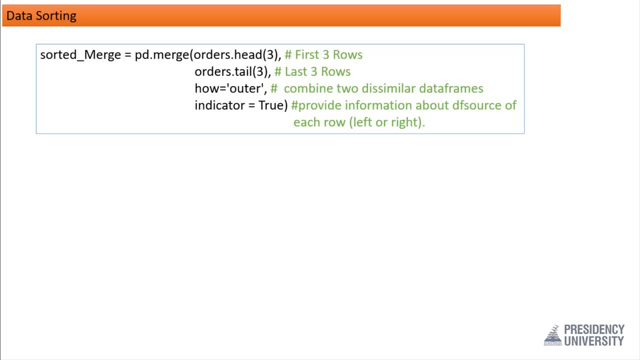 The orders dot head is going to take the first three rows and the orders dot tail is going to take the last three rows. and the how is equal to outer is used to combine the two dissimilar data frames. The indicator parameters is set to true to provide information about the data frame source. 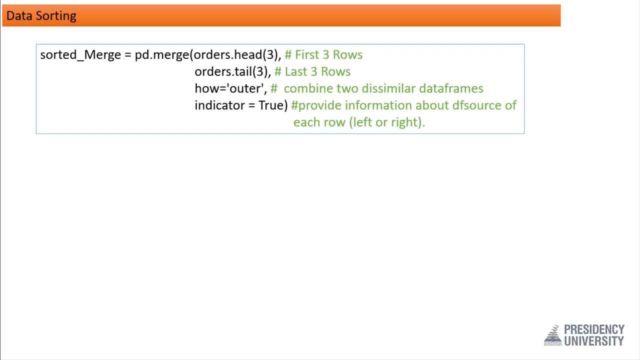 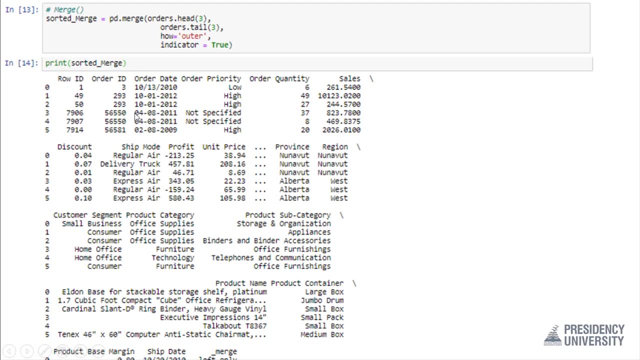 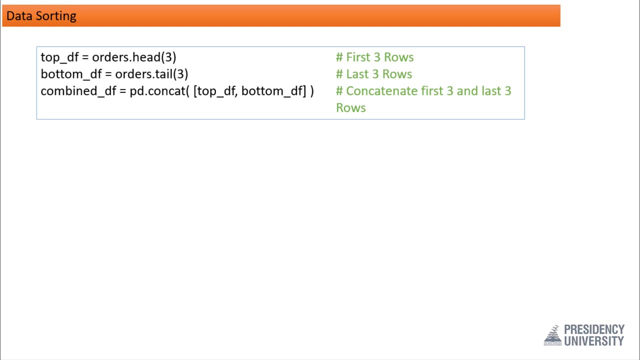 of each row to be left or right. So this enables us to merge the first three rows data and the last three rows data. this can be visualized with the row id. now let's look into concatenation. i use the dot head method to take the first three values and assign it to a variable called top underscore, df and i. 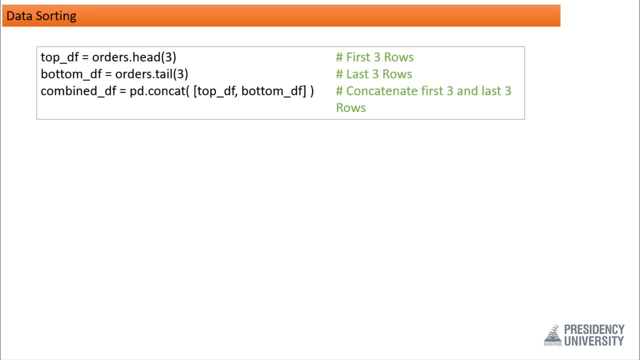 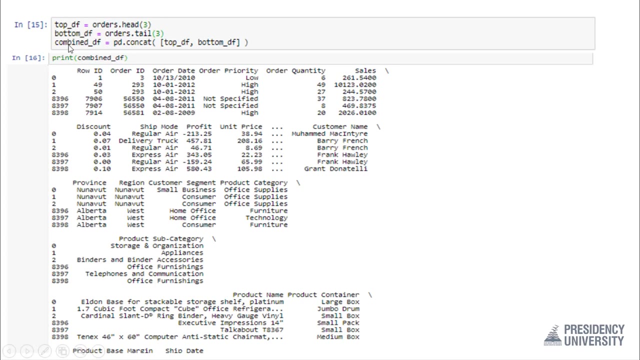 use the orders dot tail method to take the last three rows and i put it into bottom underscore df. now i use the dot concat method to concatenate the first three rows and the last three rows and i'm going to assign this to a new data frame called combine underscore df. so you can visualize. 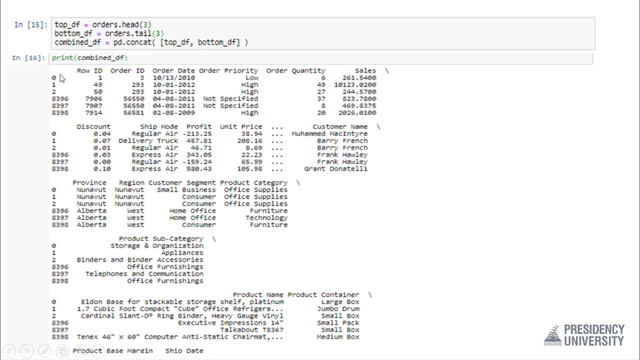 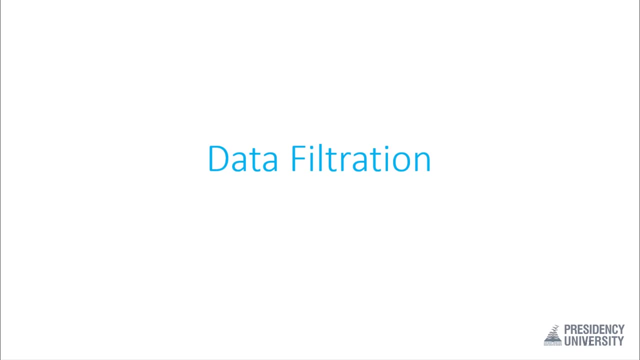 when i print this combine underscore df, i'll be able to visualize the first three rows and the last three rows together as a new data frame. data filtration is the process of filtering the data based on a given condition or as per our requirements. let's see the different cases. 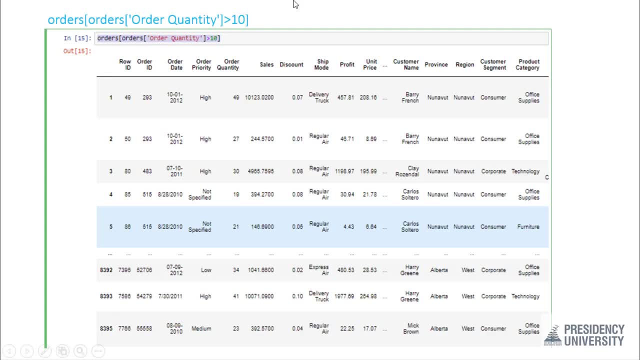 of data filtration. i take the case of this column called order quantity. here i see that the values are integers. i want to filter out the values which are greater than 10.. in order to do this, i first specify the name of the data frame. here, orders is the name of the data frame and orders of order quantity is the. 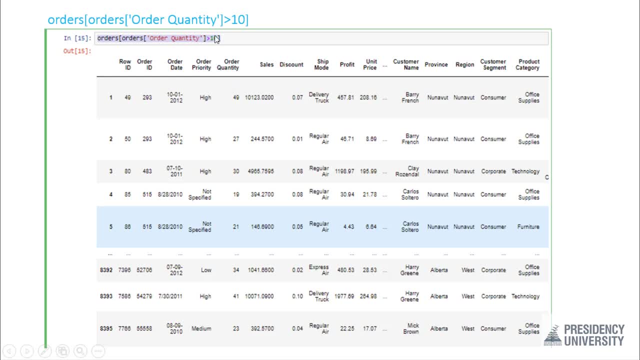 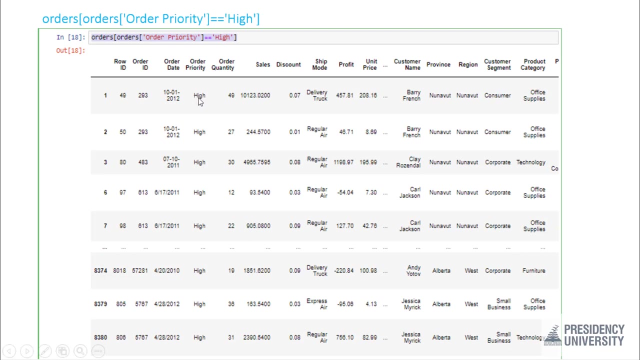 name of the column, and i have the condition here, which is that i want to filter out the values which are greater than 10, and doing so will give me the value of the data frame, and i want to also give me the values which are greater than 10.. in the next case i have a string, i have values. 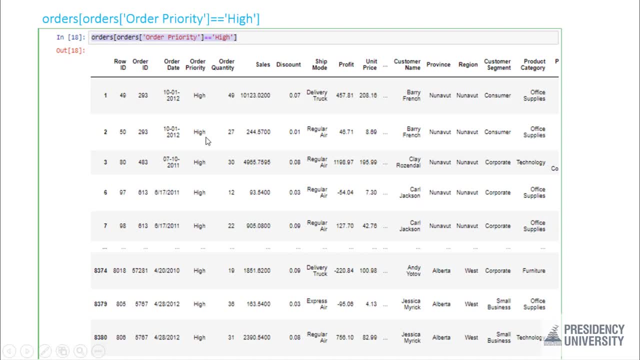 with an order priority where values are high, low in the data set. so if you want only the values which have ordered priority to be high, i can specify that to be high. so if you see here, orders is the name of the data frame, orders of order priority is the name of the column and i have 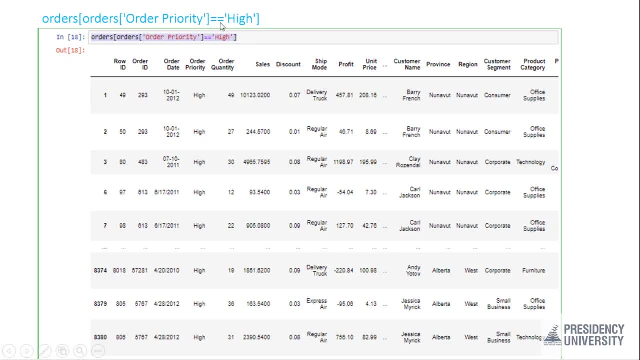 set the values i have set. if- uh, i'm checking here for equality- and if the value set is high, it will sort. only those values or those rows only alone will be displayed. In the next case I check for multiple parameters, So I'm combining the previous two. 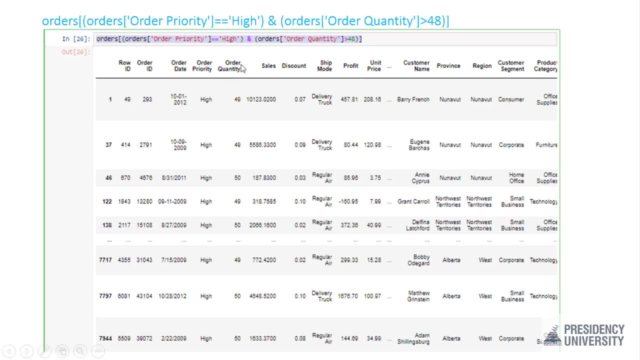 slides, wherein here I have said the order quantity should be greater than 48 and the order priority should be greater, is equal to high. So in this case I have set the orders as the name of the data frame. Orders of order. priority is the first column name, and I want these values to be high. 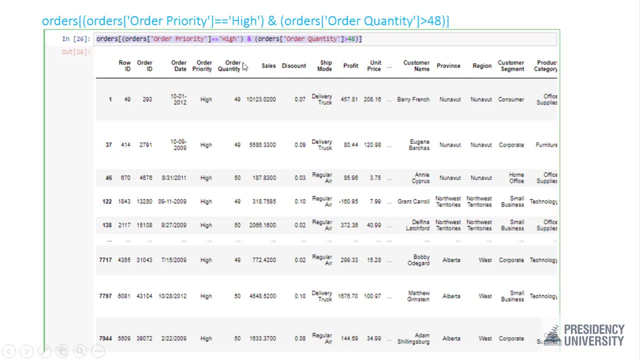 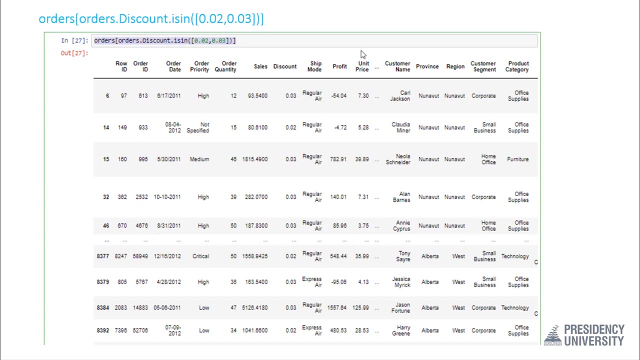 and orders of order. quantity is the second data frame and I want these values to be greater than 48 and I have split this with an and symbol. Pandas uses and symbol and not ant as in Python. The isin method in pandas library is used to check whether the specified values are in the data frame. 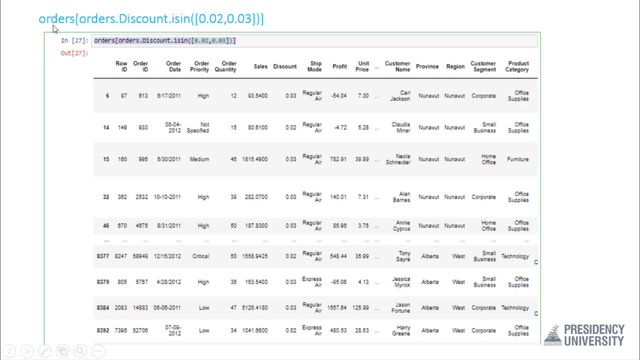 and and the isin method in pandas library is used to check whether the specified values are in the data frame and filter the values. So here we see that orders is the name of the data frame and ordersdiscount is the name of the column or the feature, and we are going to check and filter out the values 0.02. 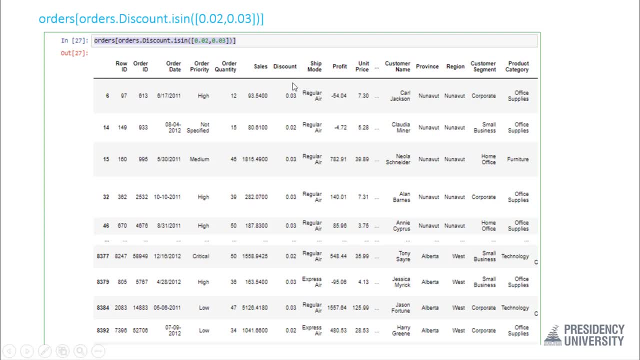 and 0.03 only. So if you see that rows which have the values to be either discount, to be either 0.03 and 0.02 are alone filtered from the entire data frame, After cleaning the data and doing the basic grouping and filtering, you may find sometimes that the values are not in the data frame. So 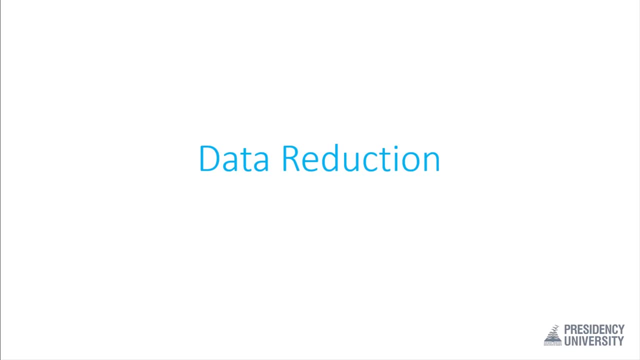 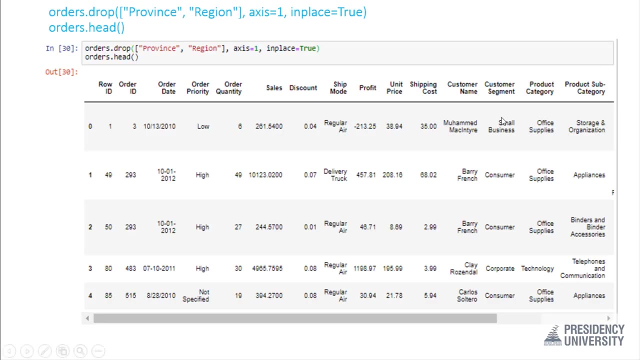 when we do this, we notice that some data or some columns are not required and hence they can be removed. Not to do that, we use the drop method. So this drop method is used to specify which columns have to be removed, And here we have used ordersdrop method, and province and region are: 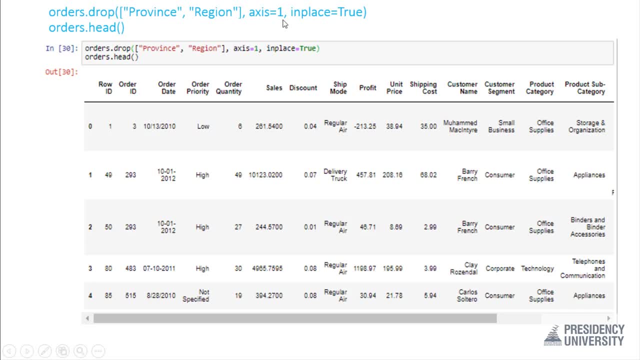 going to be removed in this data frame and we set the axis to be one and in place to be true And we display the ordershead and we see that the province and region are going to be removed. columns are removed from the data frame. Next, we are going to group the data based on the feature. 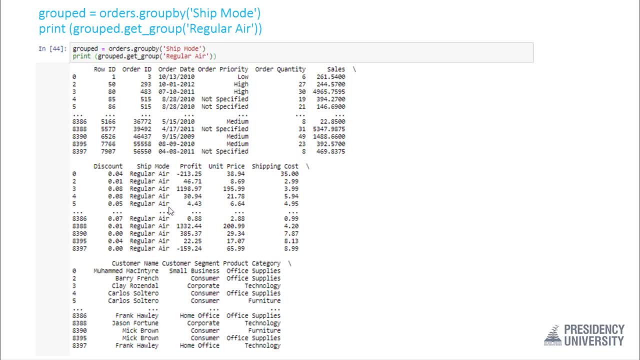 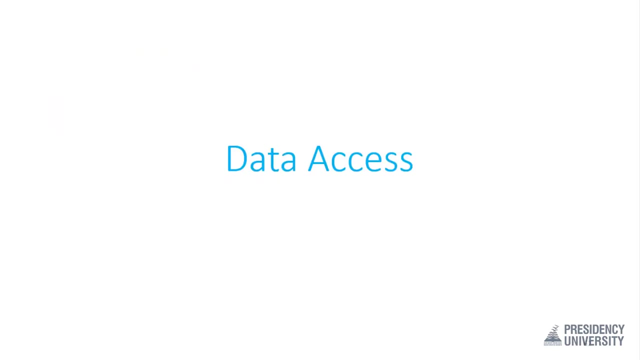 name or the column name. Here, ship mode is the name of the column and it has different parameters and we are getting the group by the parameter called regular year. So, based on this parameter, the data is being grouped. Data access: Now we are going to see some methods for data access. 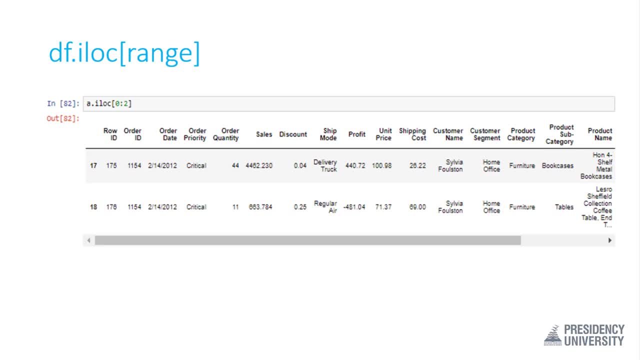 from a data frame, ILOG. The ILOG method is purely an integer location based indexing for selection by position. The inputs which are allowed in the ILOG method are integers. For example, we can put value like five, So it takes five elements or a list of array elements, or you.